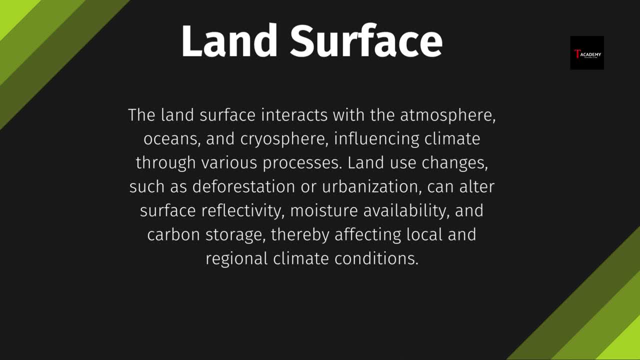 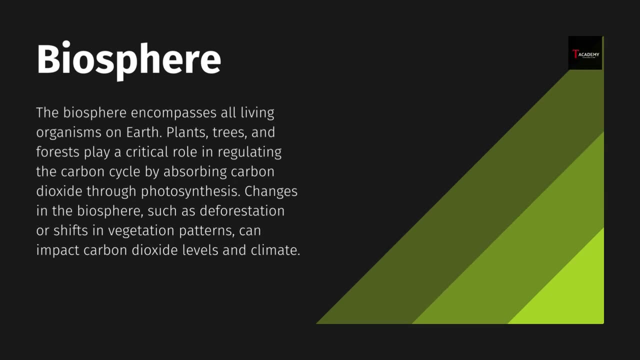 influencing climate through various processes. Land use changes, such as deforestation or urbanization, can alter surface relationships. The atmosphere is the layer of gases that control reusability, reflectivity, moisture availability and carbon storage, thereby affecting local and regional climate conditions. 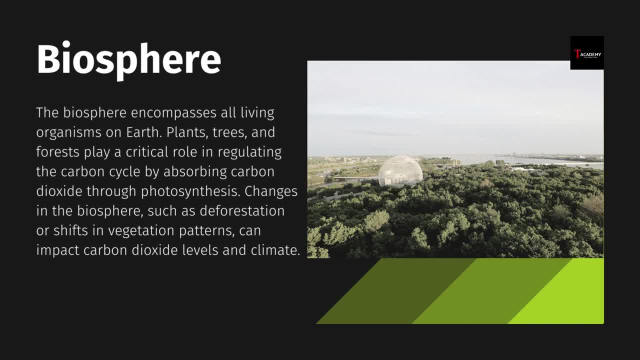 The biosphere encompasses all living organisms on earth. Plants, trees and forests play a critical role in regulating the carbon cycle by absorbing carbon dioxide through photosynthesis. Changes in the biosphere, such as deforestation or shifts in vegetation patterns, can impact carbon dioxide and the environment. 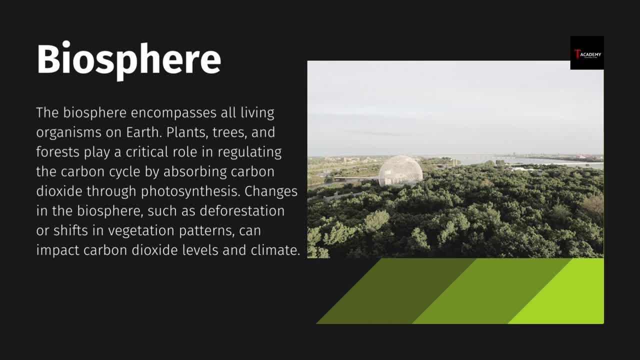 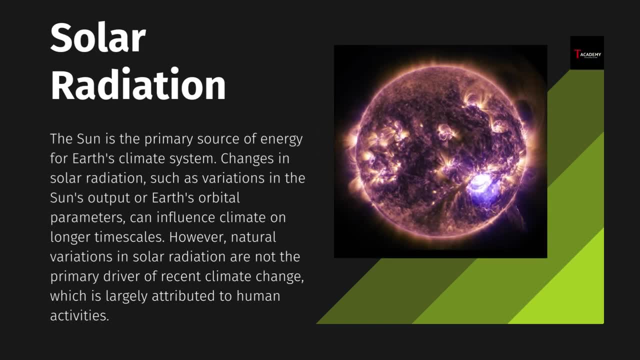 In the same way, the atmosphere is the layer of gases that control the climate. The atmosphere is the layer of gases that control the climate levels and climate. The sun is the primary source of energy for Earth's climate system. Changes in solar radiation, such as variations in the sun's output or Earth's orbital parameters. 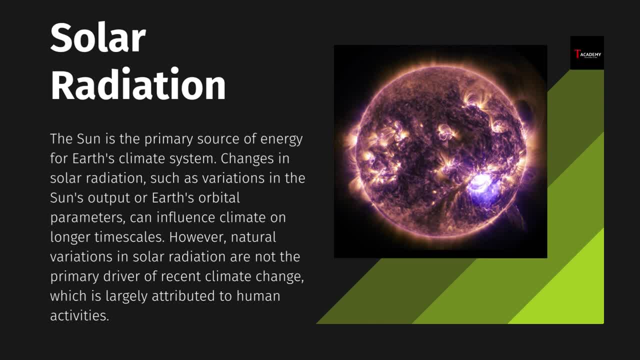 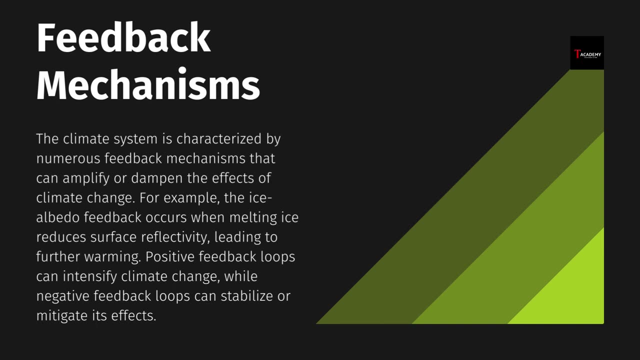 can influence climate on longer timescales. However, natural variations in solar radiation are not the primary driver of recent climate change, which is largely attributed to human activities. The climate system is characterized by numerous feedback mechanisms that can amplify or dampen the effects of climate change. 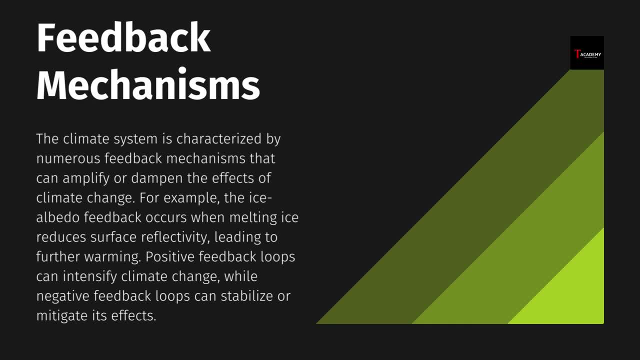 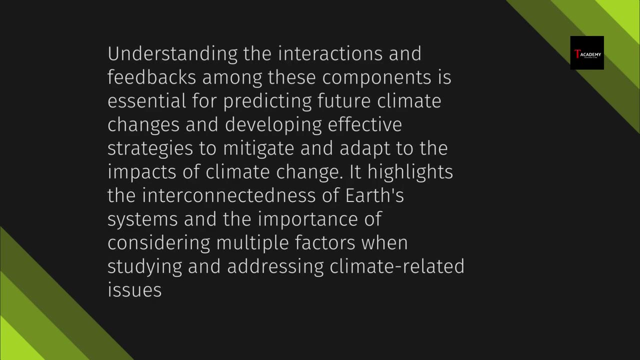 For example, the ice-albedo feedback occurs when melting ice reduces surface reflectivity, leading to further warming. Positive feedback loops can intensify climate change, while negative feedback loops can stabilize or mitigate its effects. Understanding the interactions and feedbacks among these components is essential. 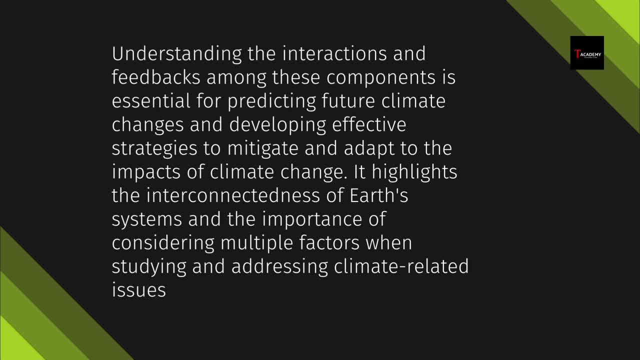 For predicting future climate changes and developing effective strategies to mitigate and adapt to the impacts of climate change. it highlights the interconnectedness of Earth's systems and the importance of considering multiple factors when studying and addressing climate-related issues. Thank you for watching our lecture on the components of the climate system. 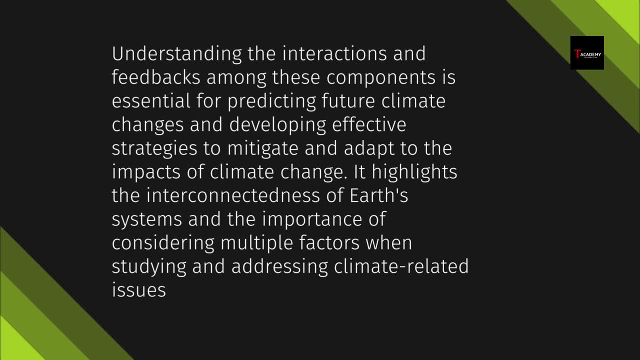 We hope you found it informative and gained a deeper understanding of how these components interact to shape Earth's climate. Remember, taking care of our planet is important. Thank you for watching our lecture on the components of the climate system. We hope you found it informative and gained a deeper understanding of how these components 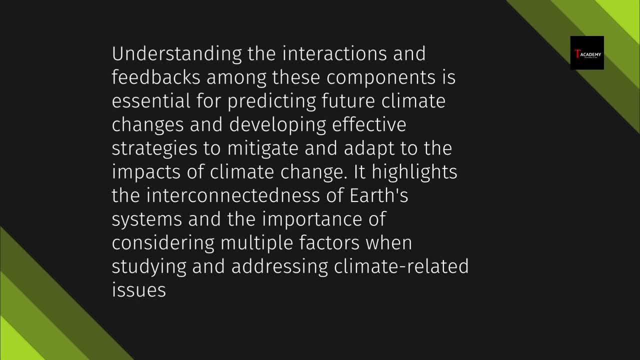 interact to shape Earth's climate. Remember, taking care of our planet is important. Take care of our climate is a collective responsibility. Let's work together to protect and preserve our environment for future generations. If you have any further questions or would like to explore more topics, feel free to.